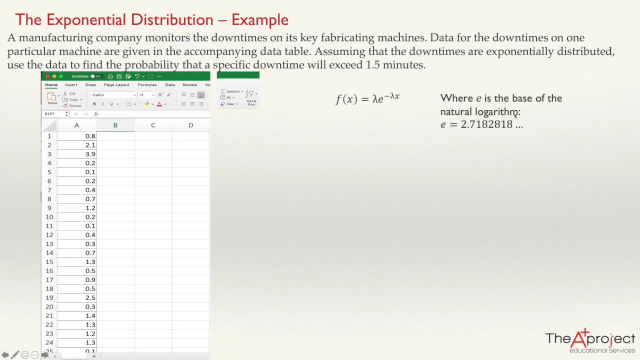 So we know that e is the base of the natural logarithm And this lambda is equal to one average of the variable. And in this problem, the variable is the down time. We need to get this average, to get this lambda, And we have the values of the down time. 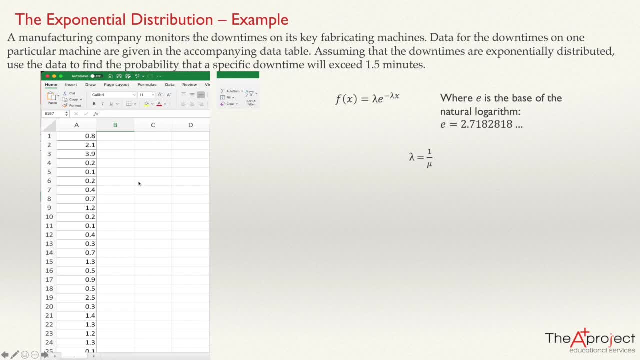 So for that reason it will be easy to compute this mean, So the mean. so we need to get the mean of all this data. Let's see how many data we have. So far. we have here until 24.. But we have more data. 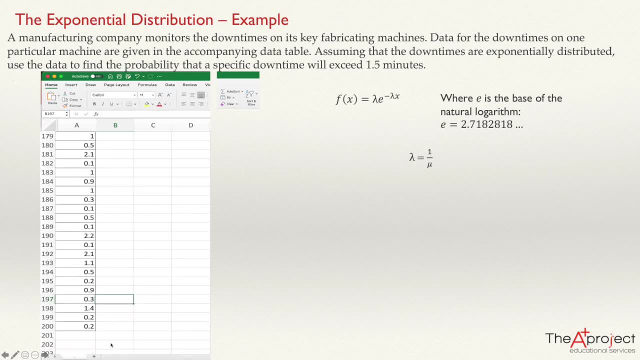 Let's see 101,, 106,, 140, 200 data. So we need to get the average of this 200 data And to get the average we can select one of the cells. Let's select this last cell here. 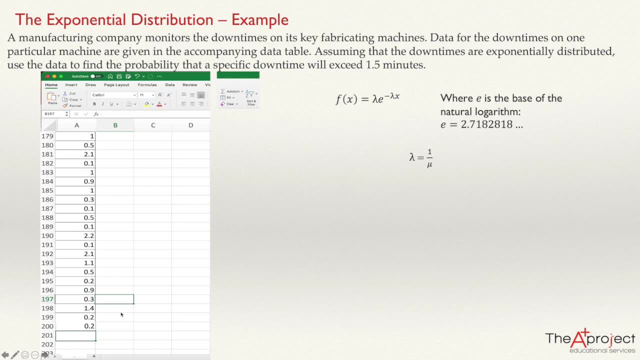 The cell A201.. We select it and then go here to autosum, Click on autosum and choose average. When you choose the average, by default Excel tells you, asks you: are you going to compute the average between cell A1 to A200?? 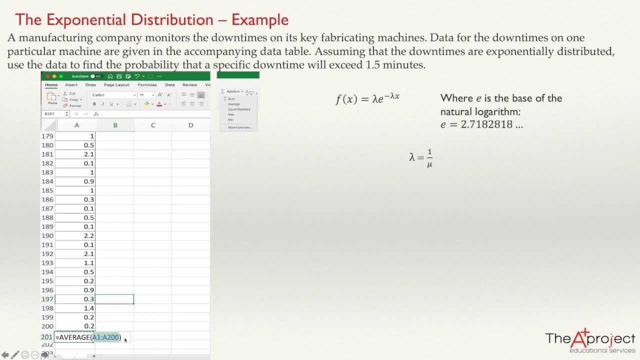 And that's true. It's between the first and the last cell of this. Just press enter and you get the average. It was 0.7085.. So you got this average And if you got this average, you're going to have 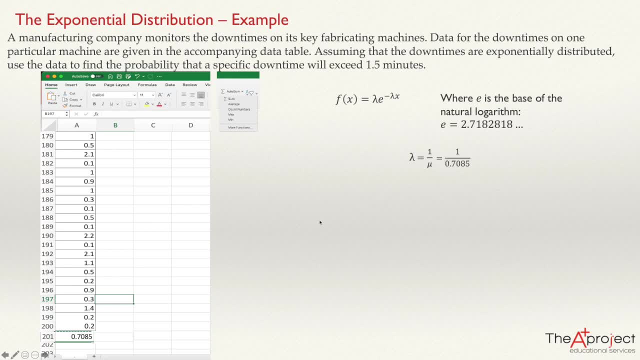 lambda. So lambda will be 1 divided by this 0.785.. So in this case the average will be 1.4114 326.. So we know the value of lambda. So now we have an idea of how is the distribution. 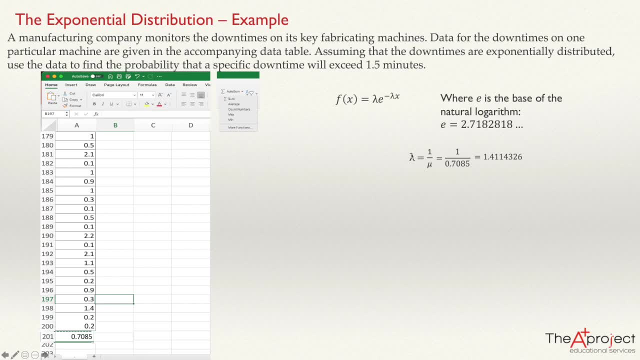 Remember that this lambda is actually give you the intersection with the y-axis And the distribution is a decreasing distribution. So it will be something like this And this number here in the intersection will be 1.4114.. Let's type here that this is. 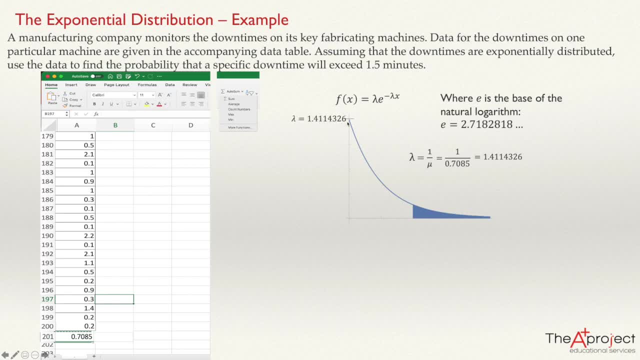 lambda equals 1.4114 326.. And here in the x-axis is the variable, in this case the downtime, that the average is 0.7085.. And I'm asking you, what is the probability that this variable is greater than 1.5 minutes? 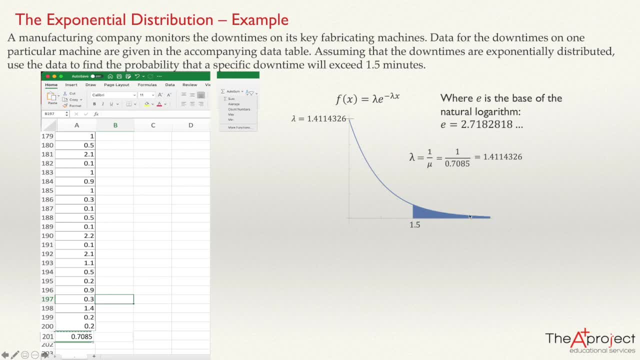 So 1.5 will be in one part and I'm asking you for this area. The average is 0.7085.. So this average will be here. So around here Let's type here: this is 0.7085.. 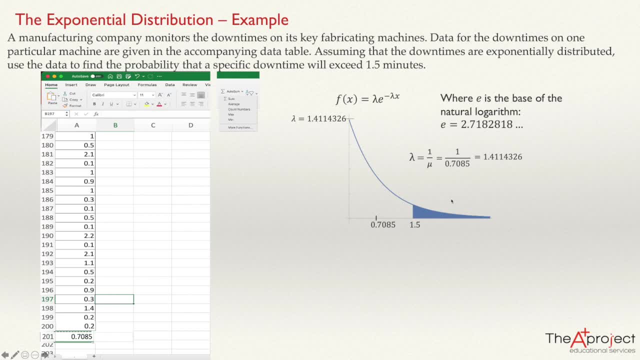 And we have a formula for the probability that the random variable will be greater than a number. We know that this formula is the probability that x greater than a variable t, it will be e to the power minus lambda t. So this density function help me. 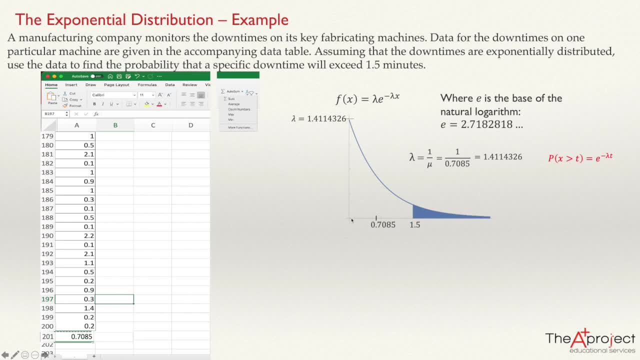 to understand how it's going to be the graph. I know that when x equals 0, so this e to the power, 0 will be 1 and lambda will be the interception. So we know, knowing this lambda, we know how is the density function. 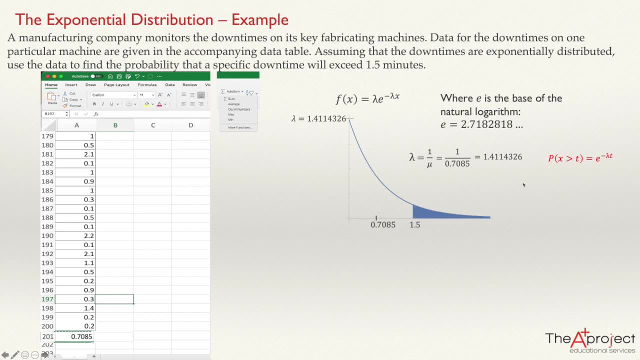 But if we want to compute the probability that the random variable will be greater than a number, we'll use this formula. It appears lambda, but just in the exponent, So let's use this formula. Now we know that t will be 1.5.. So the 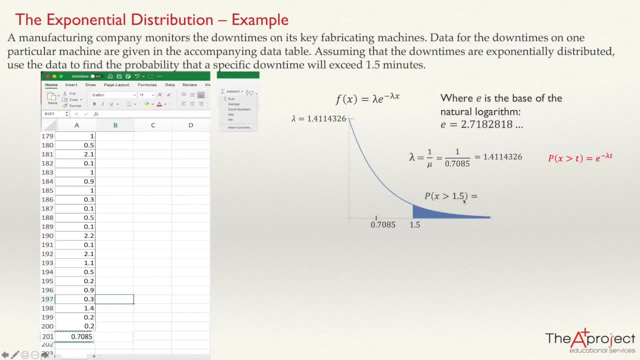 probability that x is greater than 1.5 is the question. So we are looking for this area here, You see here, And just the only thing that we need to do is just make a substitution. So here will be e to the power. 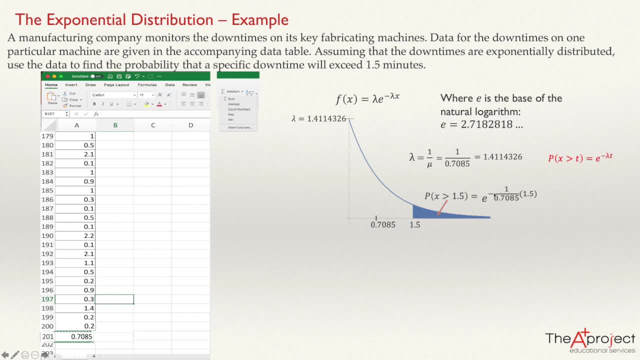 minus lambda t minus 1 over 70, 85.. You can type: lambda equal 1.4142.. 326.. But this is a rounded number, So I prefer to use the exact answer: 1 over 0.7085.. I don't want to use a rounding number here. 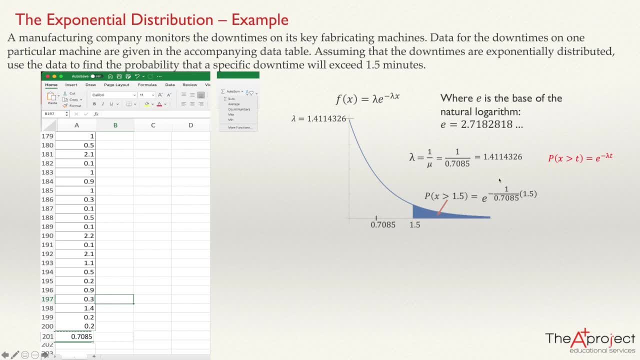 in the middle. But if you get this, if you use this, you are going to get a good approximation And multiply by t, that in this case is 1.5.. So if you are going to make this multiplication first, this 1.5 multiply 1. 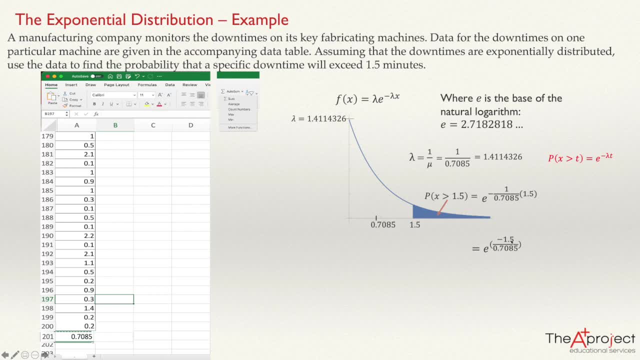 and you are going to have the power minus 1.5 divided by 0.7085.. Now it depends how is your calculator? For example, you have a financial calculator in most of them. you are going to solve this part first and then, when you have. 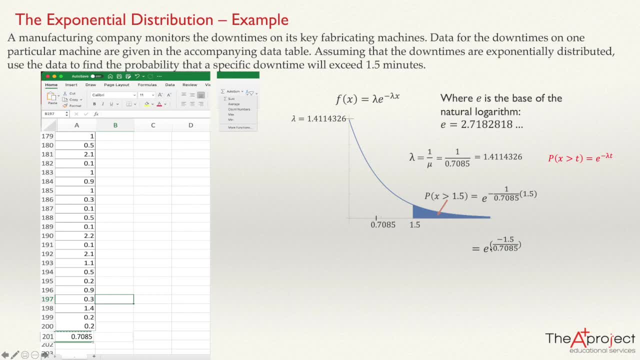 this part. use the exponential function, the e function, in your calculator, The e key of your calculator, And press equal sign. If you have a scientific calculator, maybe in the scientific calculator usually you type first the e function, open bracket and put this expression: 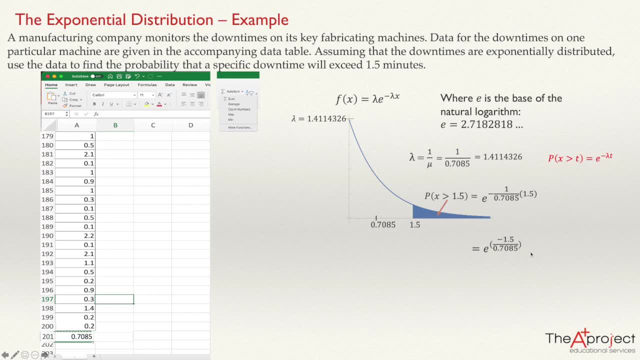 inside the bracket, cross bracket and press equal signs. So you should know how to use your calculator. Anyway, if you do that, you will get the answer 0.1204.. So this will be the probability that x is greater than 1.5.. 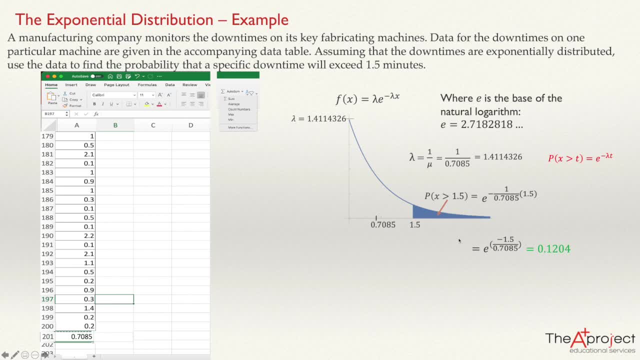 Obviously, you can solve this using Excel. If you use Excel, whatever cell of Excel, for example in this cell, you can choose this cell and press equal, but Excel knows the area to the left. If you use exponential distribution in Excel, Excel is going to give you this area. 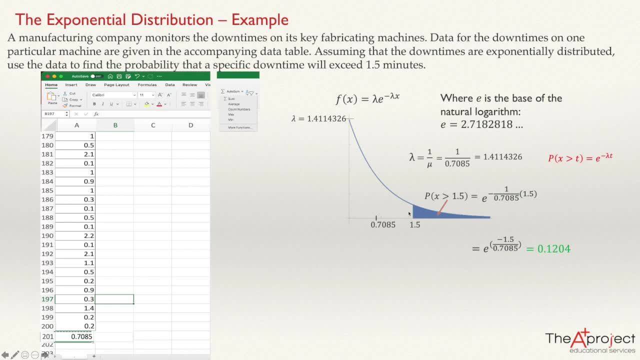 that is at the left. So you will need to do 1 minus the distribution in Excel, 1 minus the accumulated distribution, and you are going to have this area to the right. Let's do it, Let's press here: equal 1 minus. 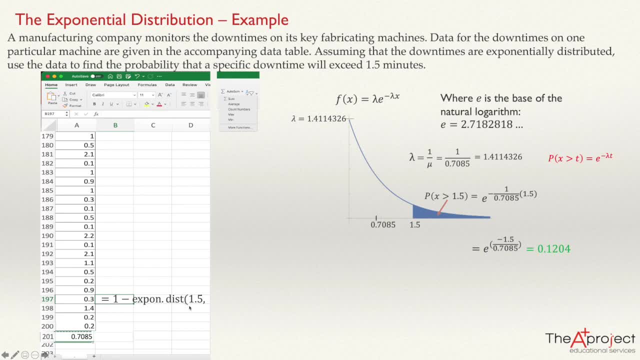 exponential distribution- open bracket. don't forget and put here the value of x, 1.5 comma, and now the value of lambda. So Excel is going to ask you for lambda And for lambda we have, that is, 1.4114326. You can also type 1. 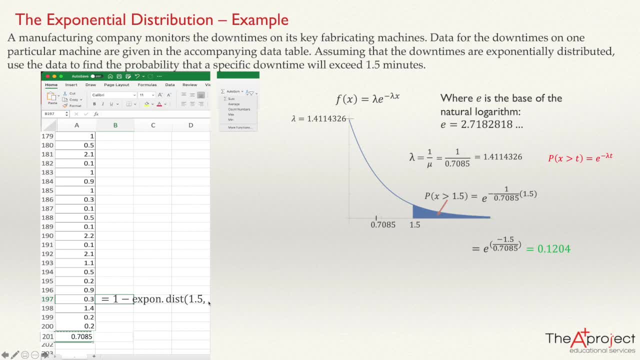 divided by 0.7085. So let's type here 1.41, 14326 comma. and now you need to tell Excel if this is cumulated or not, So you can type comma true or comma 1, and don't forget to close the bracket. 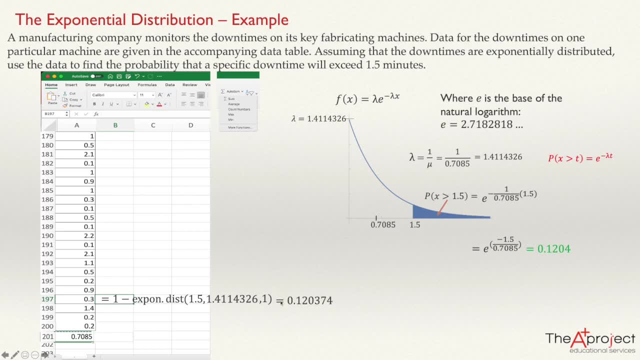 And press enter and Excel is going to give you the answer, And this obviously is the same answer that we obtained before: 0.120374, that, rounded to 4 decimal, is 4.1204 And that's it. This is the solution of this. 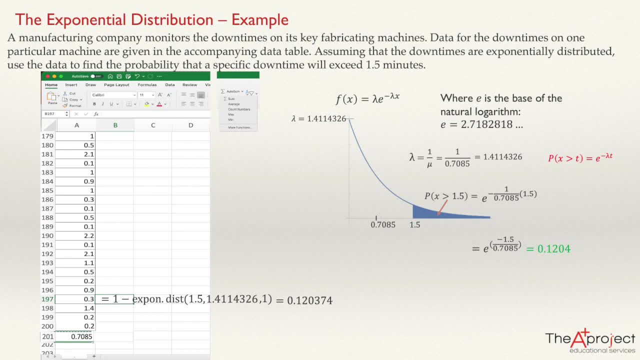 problem. I hope you can find it useful. and if you found it useful, don't forget to like, make a comment and if you haven't subscribed to this channel, subscribe to this channel. Thank you and see you in next video. 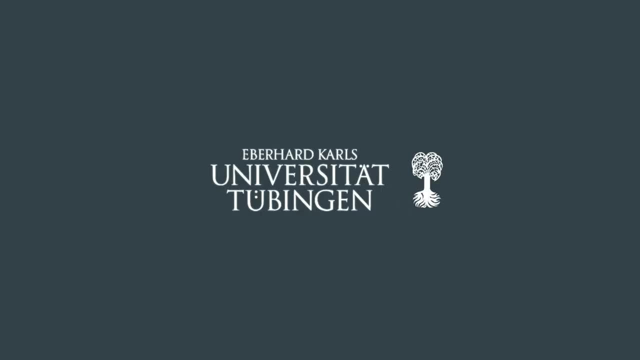 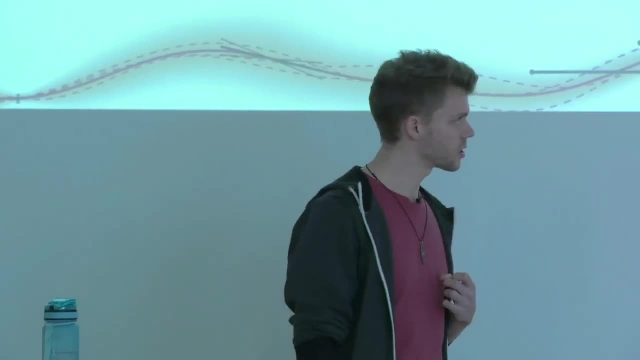 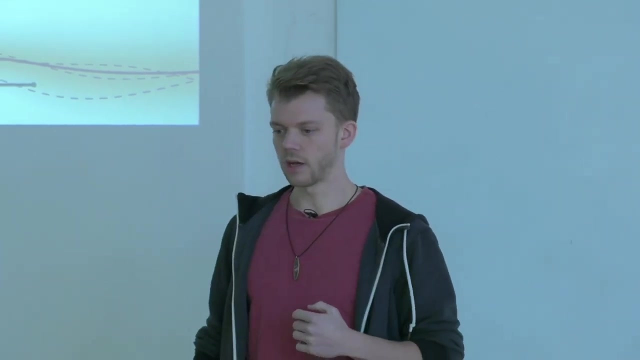 Welcome everybody to the fifth lecture of the Numerics of Machine Learning lecture course. My name is Jonathan, I'm a PhD student in Philip Hennig's group as well, and today I'm going to give you a lecture that I call States-Based Models, which we will open a new chapter. 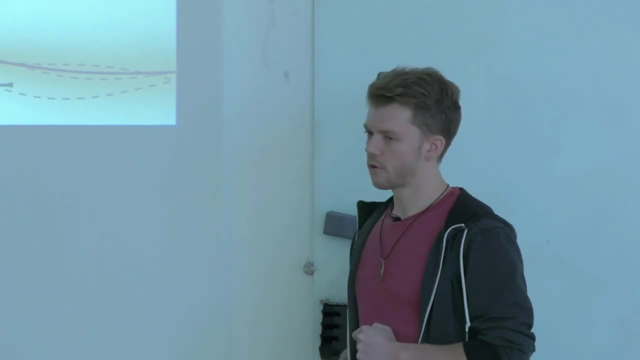 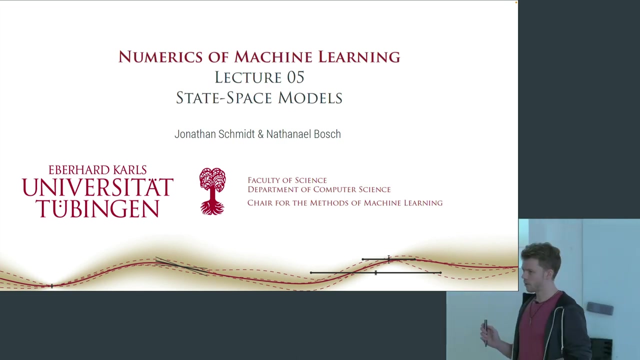 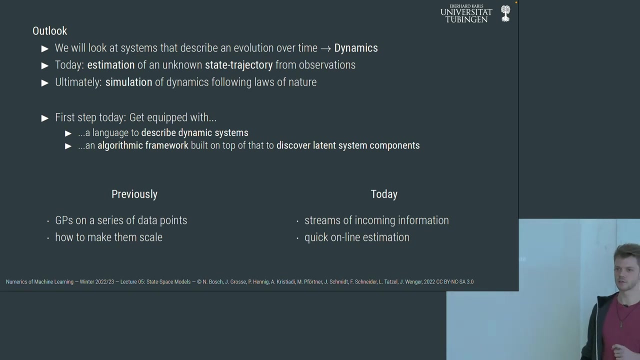 so to say, in this lecture series- and we are going to dive into a topic that is actually a very hot topic at the moment and quite emerging- What we are going to talk about in detail are dynamical systems. So over the next three or four lectures we are going to talk about systems that evolve. 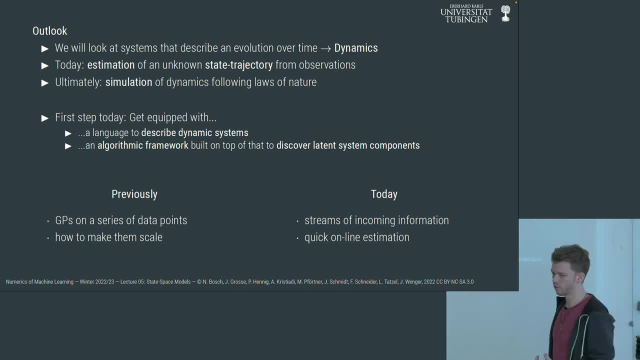 over time. This is what dynamics really means. We have an evolution over time and these systems are quite interesting. We can do a lot of stuff with those systems and today, what we are going to start off with is the task of estimating the temporal unrolling, so the temporal evolution.